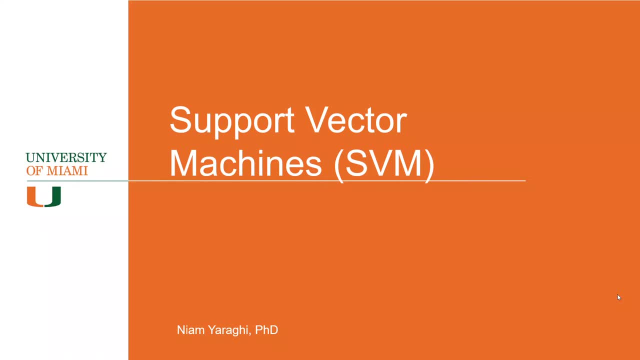 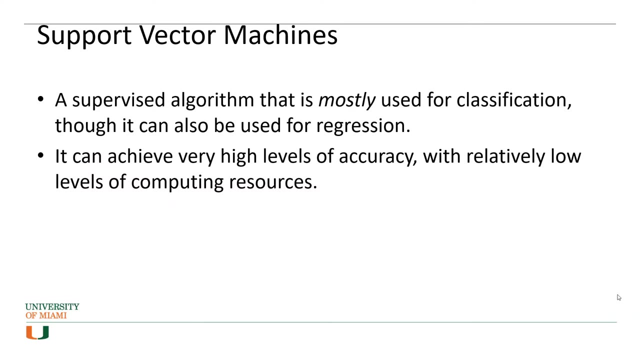 All right. in this video, I'm going to talk about support vector machines. Well, support vector machines are a class of supervised algorithms- supervised machine learning algorithms- that are mostly used for classification. However, they are also capable to do regression for you, And the good thing about them is that they can achieve very high levels of accuracy with relatively low computation power, And they are very intuitive and easy to understand. 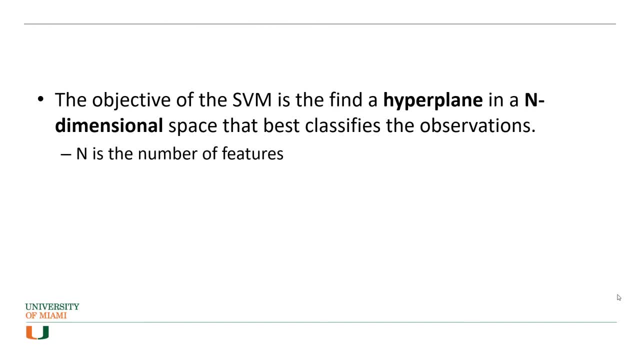 Well, the objective of support vector machine is to find the hyperplane in an n dimensional space that best classifies the observation, And here n is the number of features. Let me show you what this means with an example. So if you have a data set that only has one feature, say the age- and two classes, say whether the person is old or young, right? 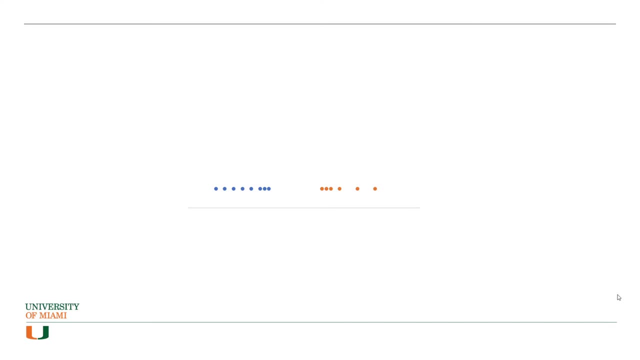 So you can have people, ages, and depending on their age, you can classify them into young and old, Here shown by the two colors, blue and orange, In this space. that is only having one dimension. the classifier is actually a point, something that is going to say: anyone who is older than this certain age is going to be considered old and otherwise is going to be considered young. Now let's say that we have two dimensions. 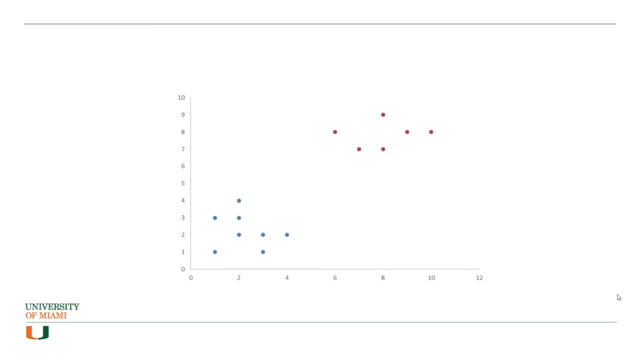 X1 and X2.. Basically, here we have two features and we have plotted our observations and used color codes in order to specify the group or the class that they belong to. Well, in this case you can find a line that is of one dimension, basically hyperplane, that goes through these observation and separates them into two classes. Anything below the line will be grouped in the classifier. 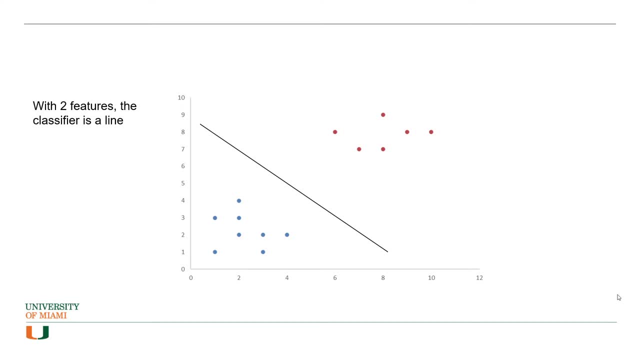 Blue class, whereas anything above the line will be grouped into the red class. Now we can extend it to three dimensions, and there you will actually have a hyperplane, and there is no limit to the number of dimensions or the number of features that you can have. The only problem is that it is going to be very difficult for us to visualize. However, the SVM works perfectly fine as you increase the number of features. 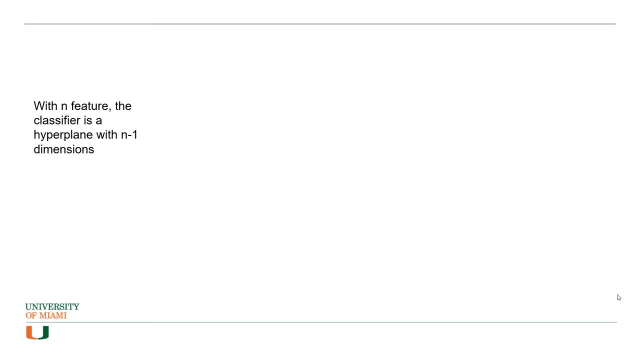 So you can generalize and say that with n features, the classifier is a hyperplane with n minus one dimensions. Now, very similar to the situation that we had with the OLS regression. we will quickly find that there are multiple lines that basically go through the observations that we have and can potentially separate them. 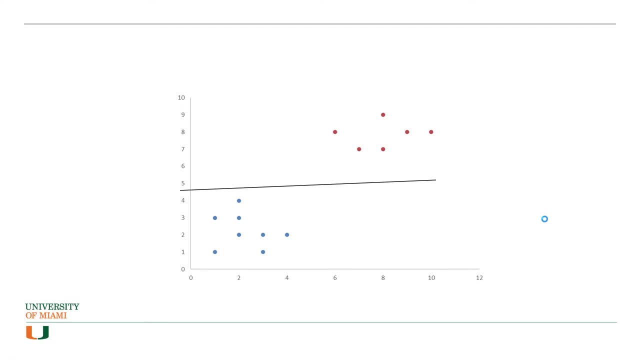 So we can generate our data into two classes, perfectly fine, at least in the training data set. And then the question is: how are you going to find the best line, Or in other words, what is the criteria for choosing a classifier? So let's start with the very first basic concept, which we know as maximum margin classifier. 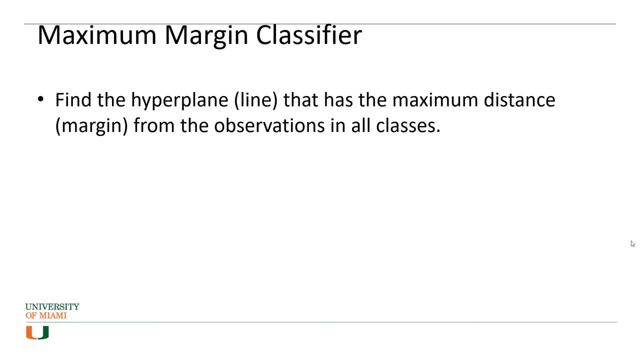 The point that I want you to remember is that the maximum margin classifier is a classifier that is a maximum margin classifier. The point that I want you to remember is that the maximum margin classifier is a classifier that is a maximum margin classifier. The point that I want you to remember is that the maximum margin classifier is very different from support vector machines, but it is the beginning of the concept of support vector machines. 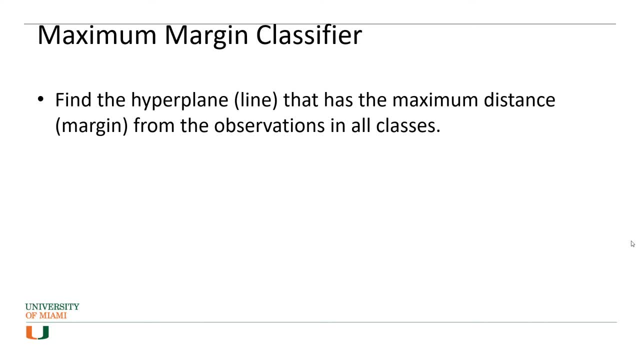 So it is very important to understand exactly what a maximum margin classifier is. All we can say that in maximum margin classifier we can find a hyperplane or, if you're talking about a two dimensions and two features data set, a line that has the maximum distance or margin from the observations in all of the observations. 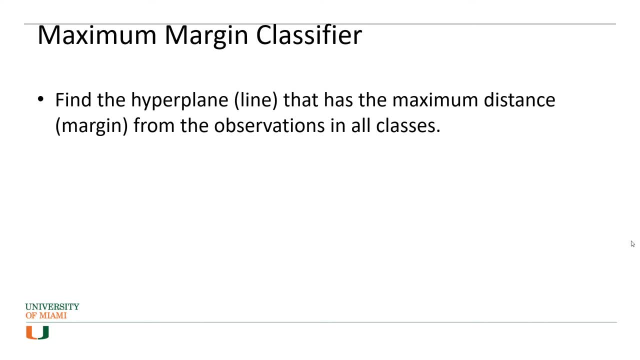 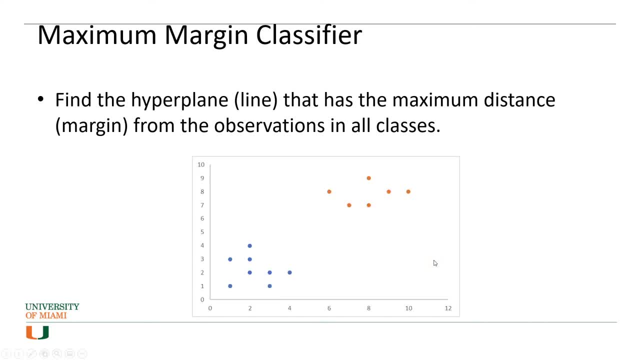 All we can say that in maximum margin classifier we can find a hyperplane or, if you're talking about a two dimensions and two features data set, a line that has the maximum distance or margin from the observations. we have basically found our line, so in this case you can say that there are multiple alternatives. 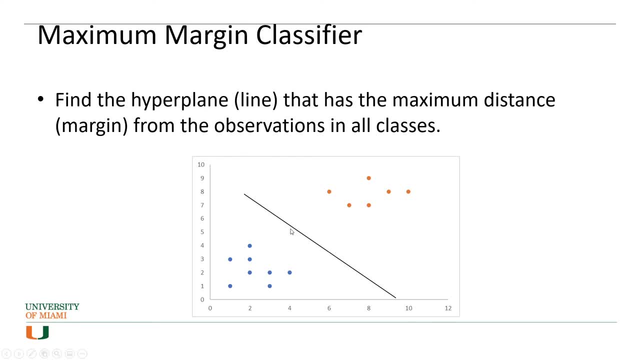 and between the alternatives, the one that actually goes right in the middle would have the maximum distance from all the observations. in other words, this line is not a really good line because it's too close to the blue class, whereas the one that is right in the middle. 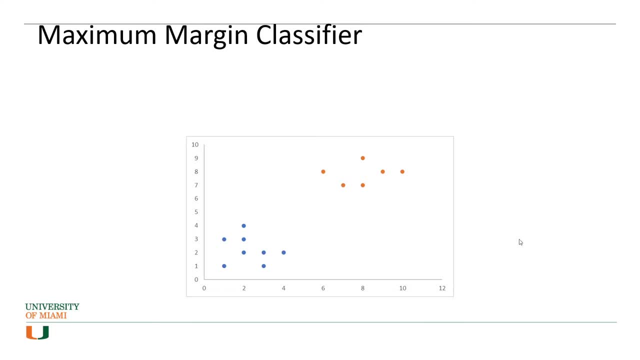 is the best one, and once we have found this line, we can say that anything that is below the line is going to be in the blue class, whereas anything that is above the line is going to be in the orange class. now let's see how it actually works. what is the mathematics behind it? well, we can. 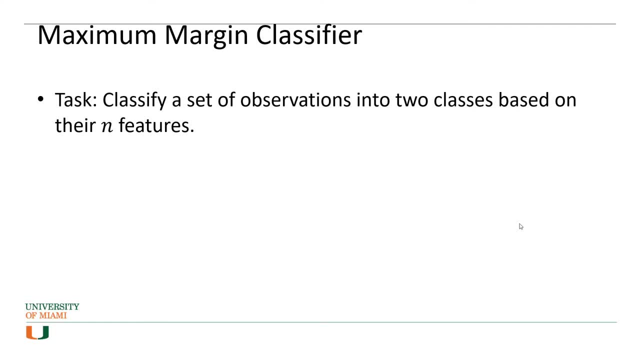 formally define the task of maximum margin classifier as classifying a set of observations into two classes, classes based on n features. Well, we can also assume that if y is equal to 1, that is denoting the observations in one class, whereas where y is equal to minus 1, it is identifying the 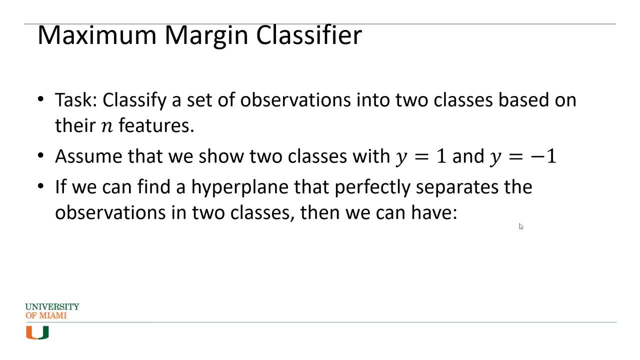 observations in the other class. all right, Now, if we have that, then we can find a hyperplane that perfectly separates the observations into two classes, such that for observations that y is equal to 1, meaning that they are in, say, the first class. 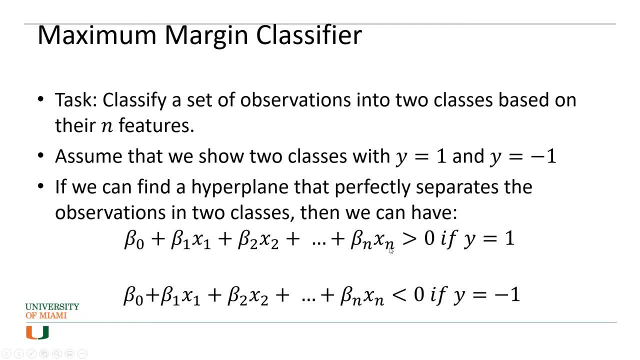 beta 0 plus beta 1 x1, all the way to beta n, xn is going to be above 0, or for observations that are in the other class, where y is negative 1,, then this equation is going to be above 0.. 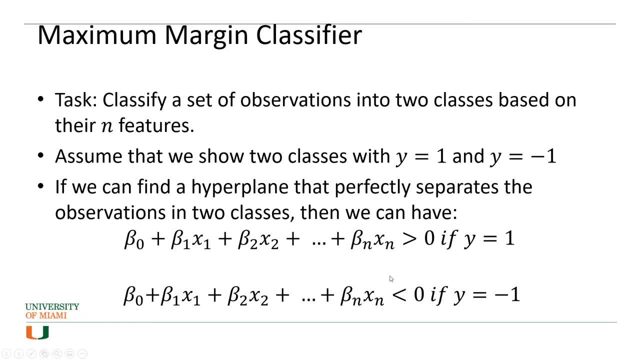 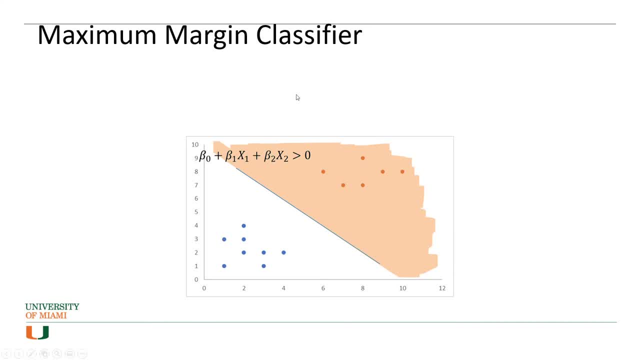 So we are going to have a value less than 0, and again, something that I want to remind you is that we are basically talking about this situation. So here, this is the formula of our line, our one-dimensional hyperline, which is saying that beta 0 plus beta 1, x1 plus beta 2: x2,. 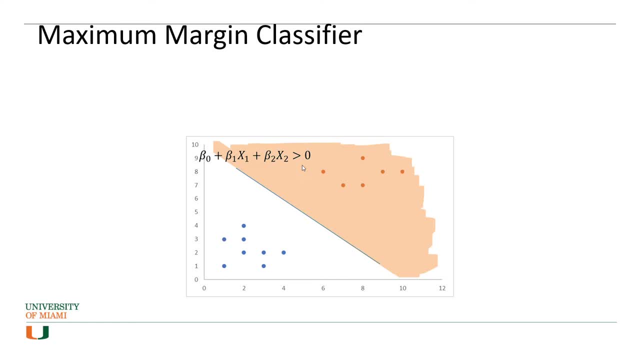 that is the formula Now. if you plug in the values of any point and that ends up being above 0, you are basically referring to a point above this line. Therefore, that is in the orange area, and vice versa If you plug in the values of any other point and that ends up being negative. 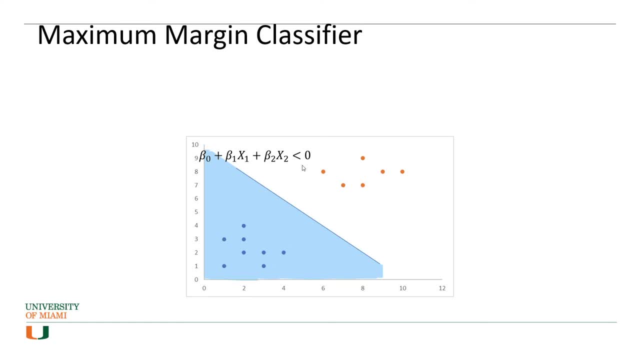 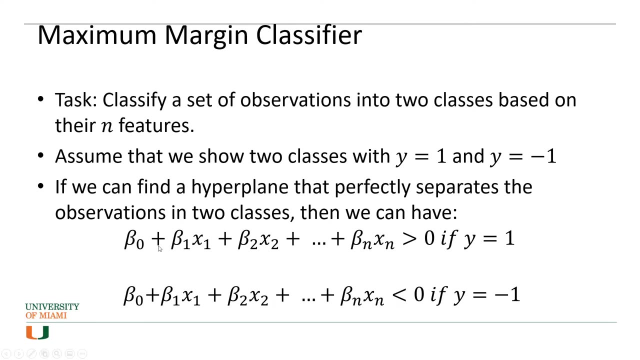 you are basically talking about a point that is below that line. So that is how this is mathematically represented. So we are going to say that if a point is in one class- say the class of y is equal to 1, if you plug the coordinates of that point into the formula of our hyperplane- 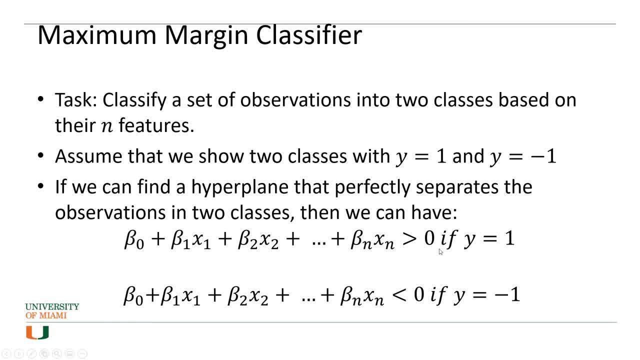 then that would result in a positive value, Whereas if the point is in the other class, if you put in the or plug in the coordinates of that point into the formula of our hyperplane, that would give us a negative value, indicating that it is in the other class. 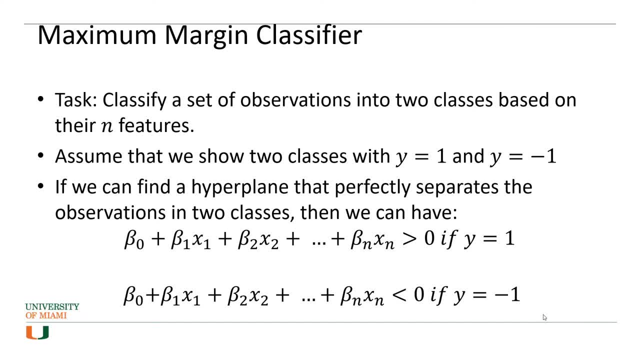 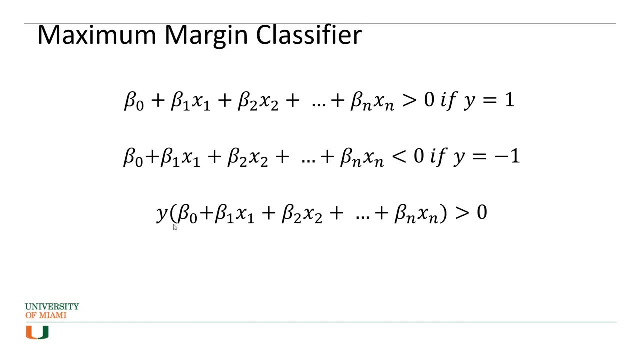 In the, or basically it is below the hyperplane. Well, with the assumption of y equal to 1 for one class and y equal to negative 1 for the other class, we can summarize these two equations into 1.. We can write them as multiplication of y by the formula of hyperplane, and then we can say: 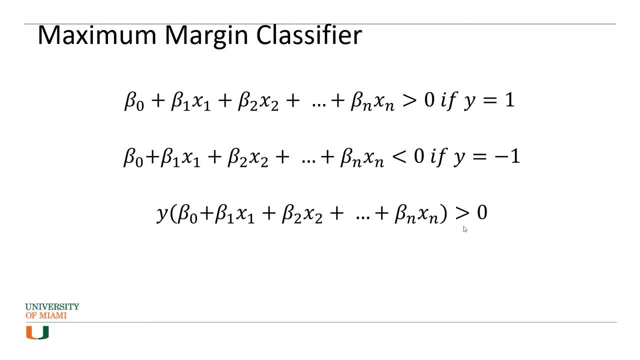 that this should be larger than 0.. Now let's see why is that? Well, for the observations where y is equal to 0, we can write them as multiplication of y by the formula of hyperplane, and then we can say that this should be larger than 0.. Well, for the observations where y is equal to 1, meaning that 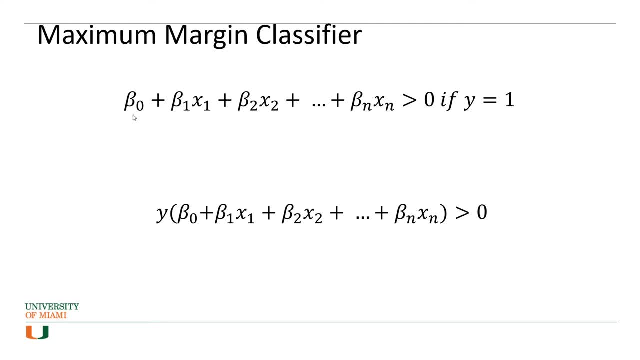 they are in our first class. we have this condition that when we plug in their coordinates into the formula of the hyperplane, the value should be positive, meaning that it should be above the hyperplane, right? So in that case you can actually say that y multiplied by this. 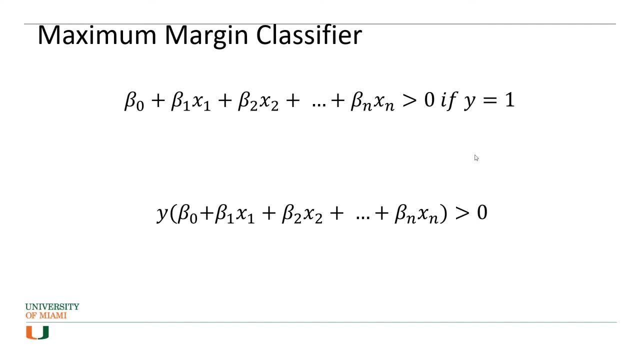 value should be something that is greater than 0,. right, Because 1 multiplied by something that is, by something that is the value of the hyperplane, should be larger than 0, and that is shown by. you know the inequality here. Now, in the cases where y is negative, 1, and this value should be. 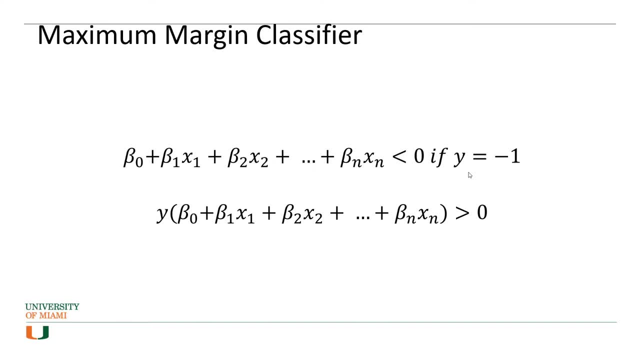 negative, then we are basically saying that if you multiply two negative values it is going to be positive, right? So you can say that the multiplication of y by the result of plugging in the coordinates of that potentially of that point into the hyperplane should be: 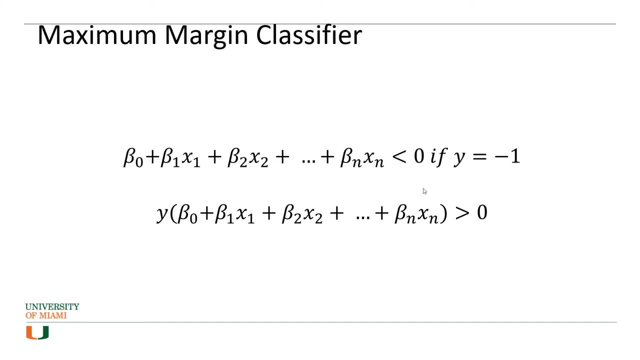 negative, and if you multiply two negative with each other, the results should be positive and therefore it is what we have shown here. So once we have summarized the classification of the observations into the two groups, using this one single formula, we can actually go. 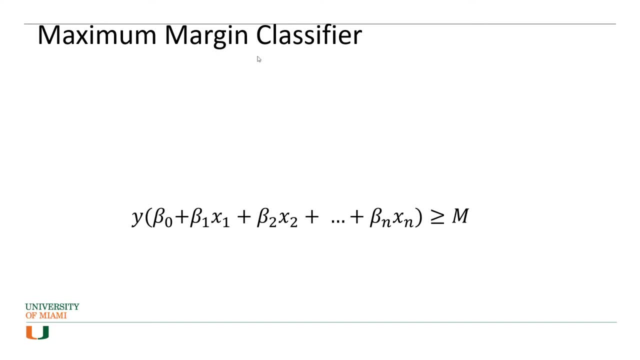 and define the maximum margin classifier as following: So instead of saying that, look, we want the observations to be either above or below the hyperplane, we can say that we want their distance to be larger or equal than m, in which m is a positive value, right? So this is. 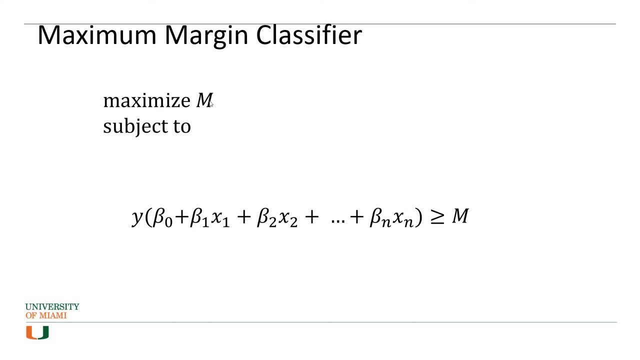 the distance, and what we want to do is we want to define the maximum margin classifier as following: So what we want to do is to basically maximize the distance, right? So we have to figure out a way in which we can maximize the distance of all the observations from our hyperplane. So that is going. 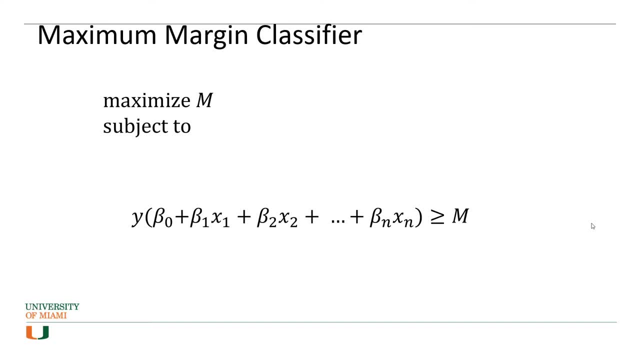 to be a conditional maximization or optimization problem, Then the other condition that we are going to have here is to say that the sum of the beta j squares should be equal to the maximum margin classifier. So what we are going to do is to say that the sum of the beta j squares should be equal. 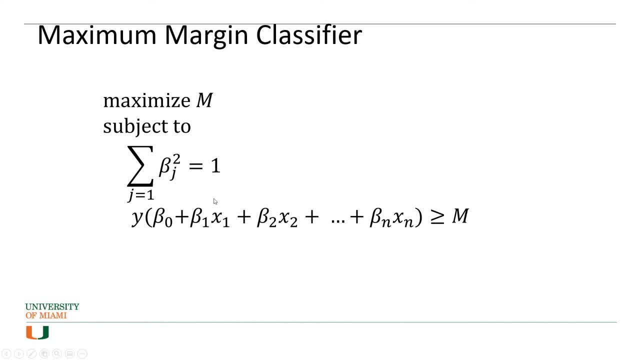 to 1, and the reason that we have this here is to give meaning to the second equation, and that is based on what I'm going to describe to you right now. So again, if you have the hyperplane's formula here- beta 0 plus beta 1, x1 plus beta 2, x2, and you want to calculate the, 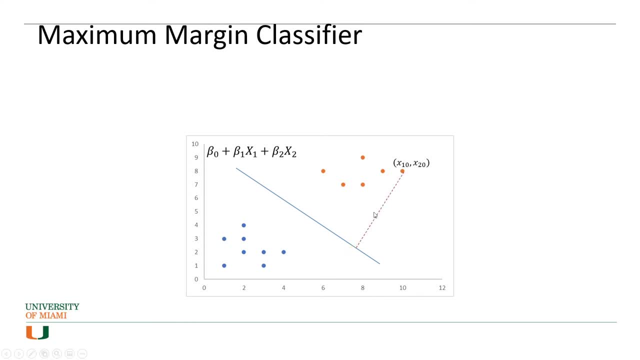 distance of any point to that hyperplane and call it d, then the distance would be equal to beta 0 plus beta 1, and then instead of x1, you're going to put the coordinates of the first dimension. Here is x1, 0, and then instead of x2, you're going to put in the 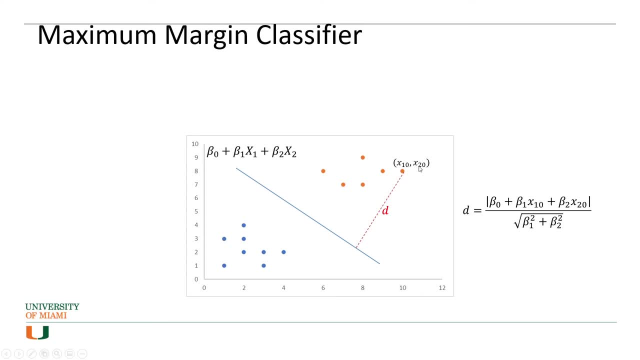 coordinates of the second dimension, which is x2, 0 here, and then divide it by the sum of beta 1 square and beta 2 square. okay, This is the- you know, formal formula for the distance between any point and any hyperplane. all right, Now, if the sum of beta 1 square and 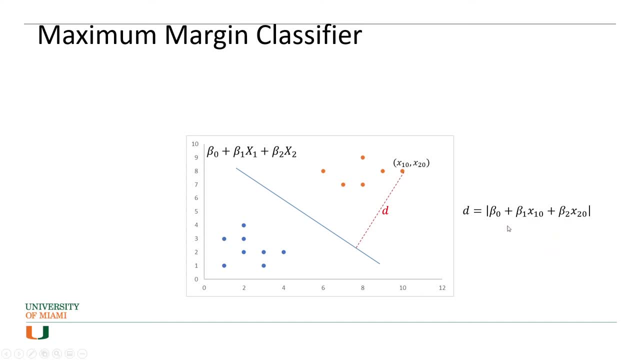 beta 2 square is actually equal to 1, then you can remove it from the denominator and say that the distance is going to be beta 1, beta 0 plus beta 1 x1 plus beta 2 x2,. right So, and that is. 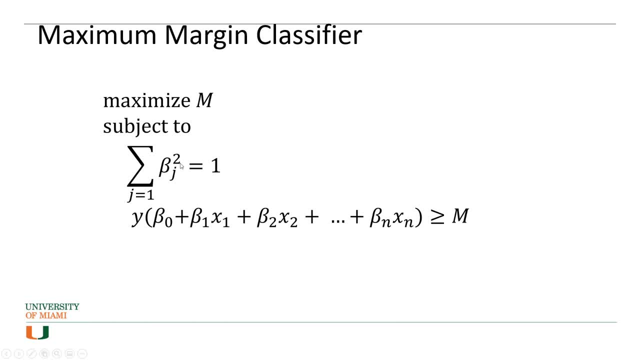 basically what we have here. If this condition is true, if the sum of the beta squares are actually equal to 1, then you can actually go ahead and say that this is the formula for distance and what you're going to do here. the task here is to maximize the distance of the hyperplane from 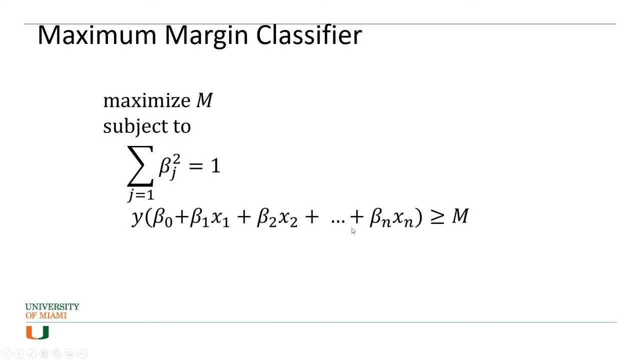 all the points in our data set, regardless of the class that they are in. So that is the conditional or constrained maximization problem that we have to solve, and it's quite easy- actually The Lagrange functions- to solve this maximization problem. 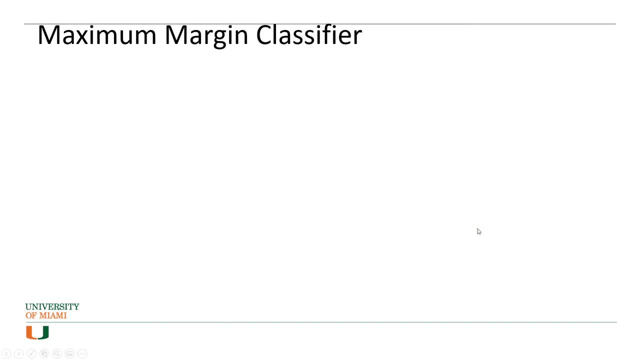 Now let me show you visually how it works. Well, let's say that we have collected data on the number of hours that students have studied and also whether or not they passed the course. So here we have one feature and two classes. The feature is the number of hours studied. 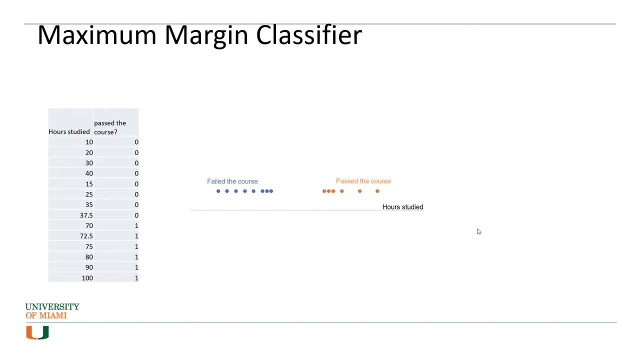 and the classes is whether they passed the course or not. We are going to show them with two colors: orange for the ones that they have studied and yellow for the ones that they have passed the course, and blue for the ones that failed the course. Well, here we can find a. 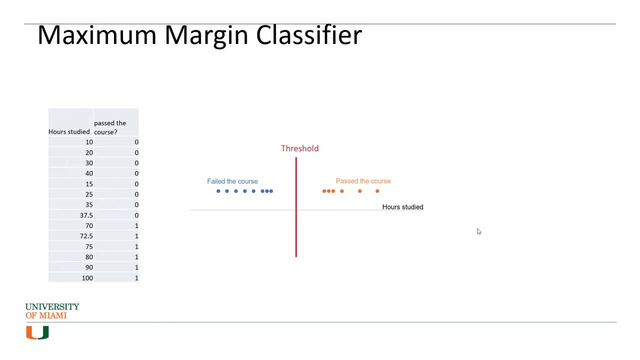 threshold here in this point is going to actually be a point that has the maximum distance from all the other observations in the data set and that is the one that I have shown here And we can actually show that that is going to be right in the middle because the threshold that 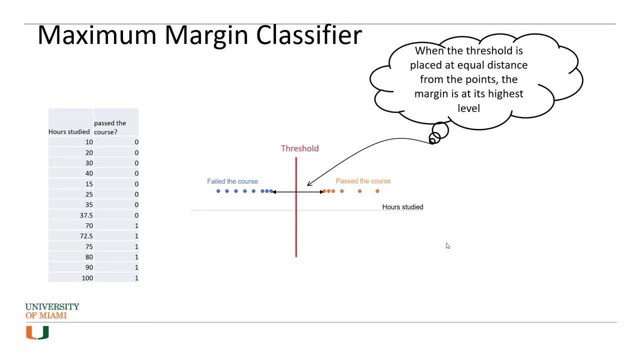 is placed at equal distance from all the points would have the highest distance from all the points, And this is basically our maximum margin classifier. So all is good now, but let's see what happens when we have some outliers in our data set. So 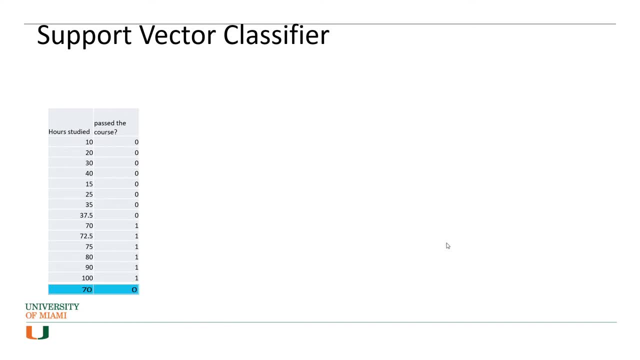 in this example. suppose that there was a new student that was added to our class who, despite studying 70 hours, ended up failing the course, and that is going to be the new visualization of our data. So we're going to have this new student with the blue dot that has. 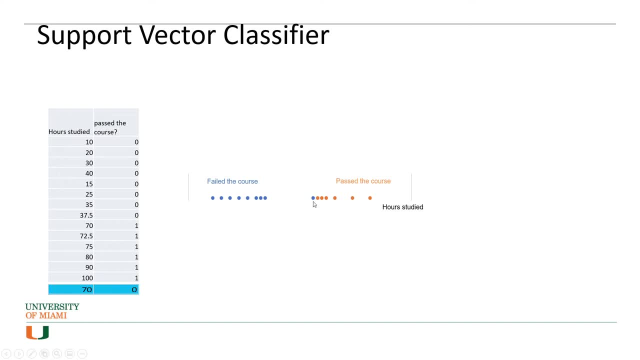 failed the course, despite the fact that the number of hours that he has studied is way closer to the students who have actually passed the course. So we're going to have a new student who has failed the course. So we're going to have a new student who has failed the course. So 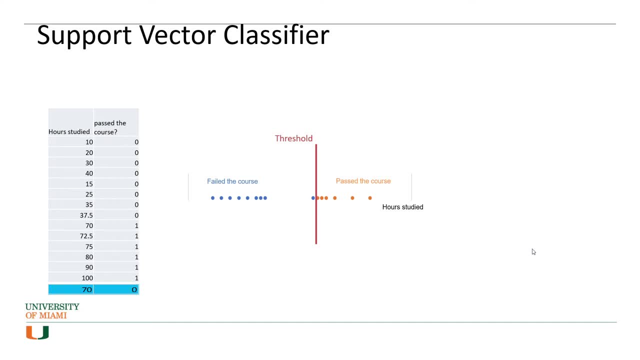 in this case, the threshold is going to be moved to the right, and that is quite a dramatic change. In other words, the classifier is very sensitive to the outliers And what happens is because of that sensitivity, when we find the classifier using our training data set. we are not going to have 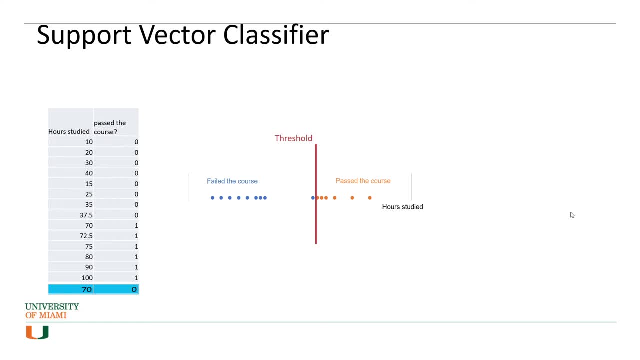 going to be able to do a good job on the testing data set. So if, for example, there was a person who had studied these many hours that I'm showing with this new, larger orange line and had actually passed the course, our classifier is going to classify it as a person that has failed the course. 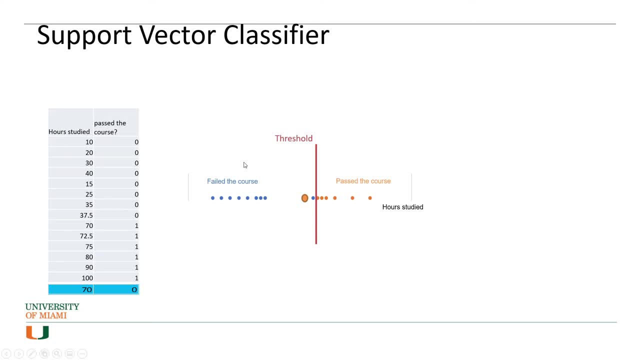 Why? Because the value is less than or is to the left of the threshold. Therefore, the classifier is going to say that this observation belongs to the group of failed student, And you know it is basically doing a wrong classification. So how can we solve that? Well, we can allow for. 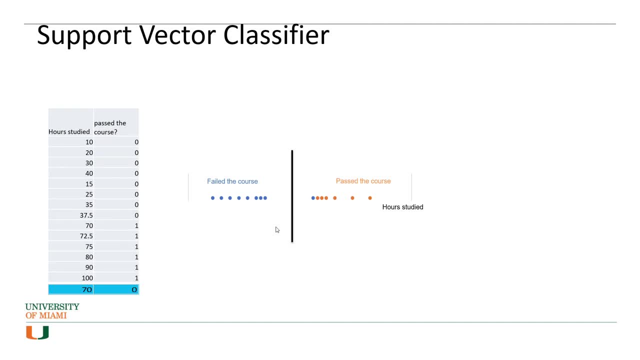 misclassification. What does it mean? It means that we go ahead and find another classifier. In this case it's actually called support vector classifier And we are going to allow for some margin of error, meaning that, hey, we are going to choose. 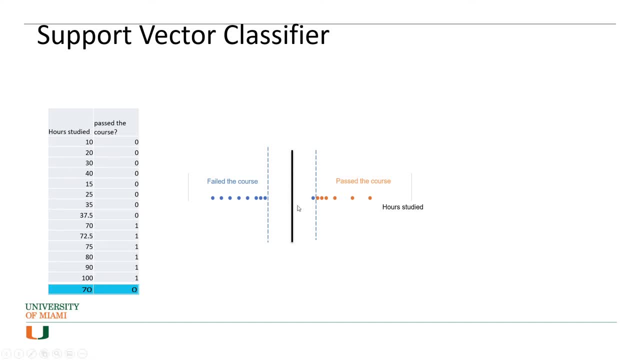 this point as our classifier, despite the fact that we know in the training we are making a mistake, right. So this blue observation should have been classified as passed, but we are. uh, should have been classified as failed, but we are. 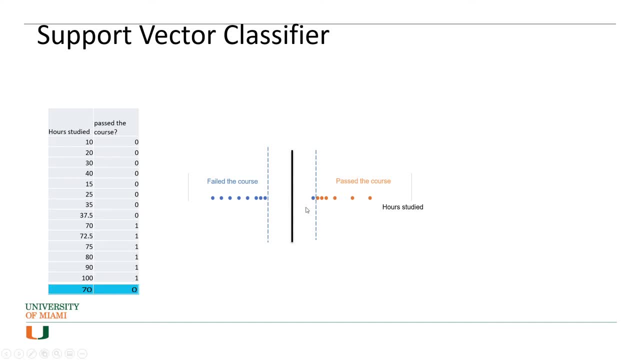 knowingly classifying as passed because it is within a margin of error. Okay, Uh. so if we do that, then rather than having like a uh, a dot, or in a two dimensional space, imagine that you have a line- uh, we are going to have a tube. It looks like a street, right That you have the. 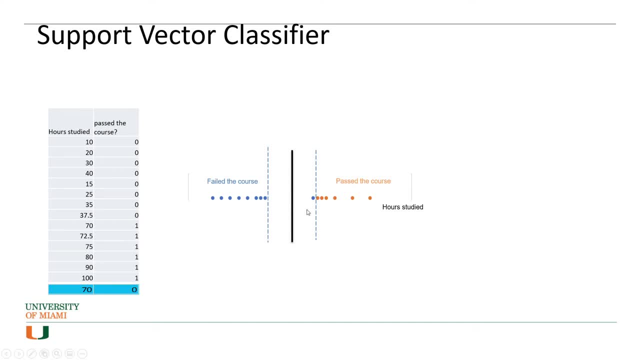 middle line and then, uh, you have two lanes, to the right and the left. So the, the, uh, the task here is to find the widest street, or or the, or the widest tube that you can run across your observations in order to classify them into two groups. uh, while accepting some level of 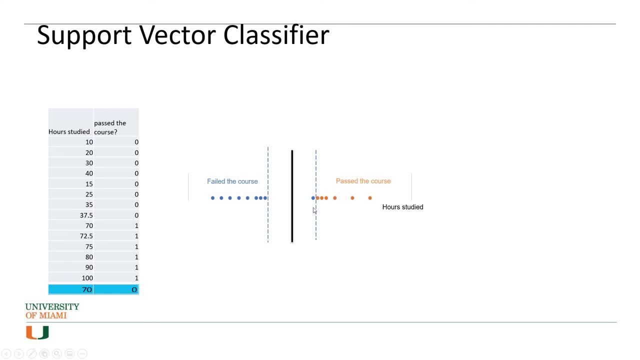 error in the training as a trade-off for higher performance when it comes to testing. And, uh, what I mean by that is that, in this situation, while in in testing, you were making an incorrect uh uh classification. uh, when it comes to sorry. 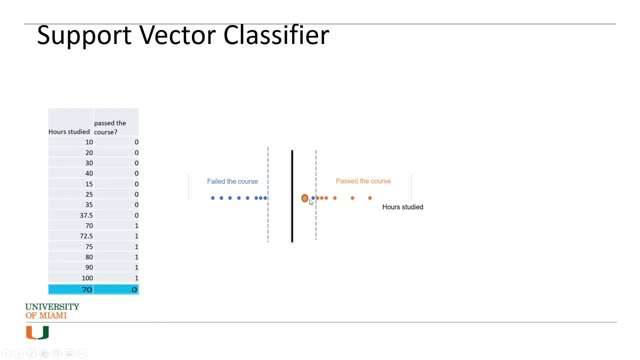 when it comes to testing, then, uh, you would be able to actually correctly classify this observation because it is to the right of your uh support vector classifier, And you would classify this person as someone who has passed the course And that is correct. So, although 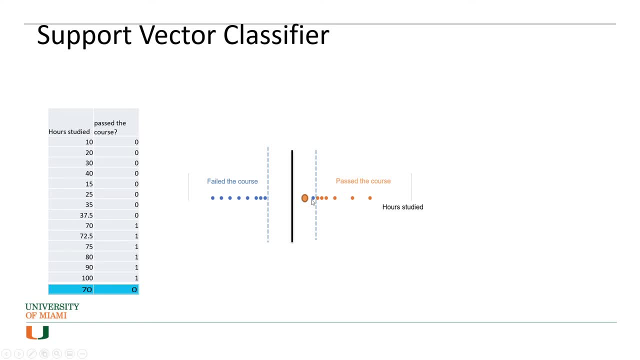 in training. you are misclassifying this blue uh orange dot. in testing. you're correctly classifying this uh orange dot Uh, to put it formally. while the new line makes some mistakes on the training data, it will perform. 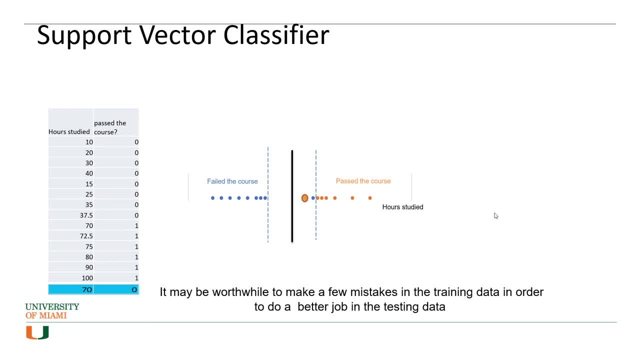 better on the testing data. Uh, and it basically may be worth to make a few mistakes in the training data in order to do a better job in the testing data. Now, the lingo here is that, the observations on the edge, uh. 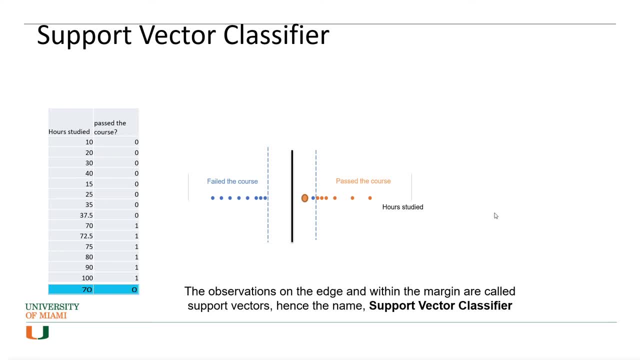 are called the support vectors and therefore the classification algorithm is called the support vector classifier. now, the other point that i want you to pay a lot of attention to here, and that is very unique about the support vector classifier and support vector machines, is that only the observations at the edge are going to affect the 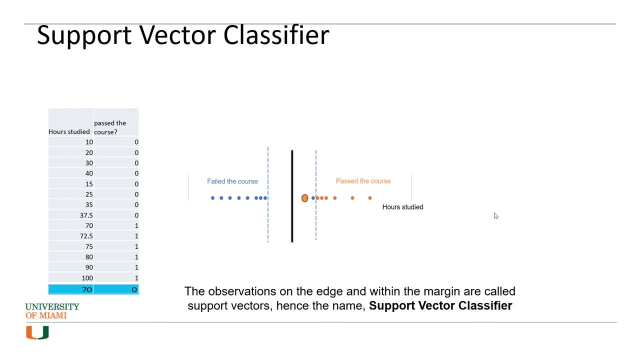 position of the support vector classifier, meaning that if you come and add many other points to the left for the students who failed the course and many other points to the right for the students who pass the course, it is not going to affect the position of your classifier. 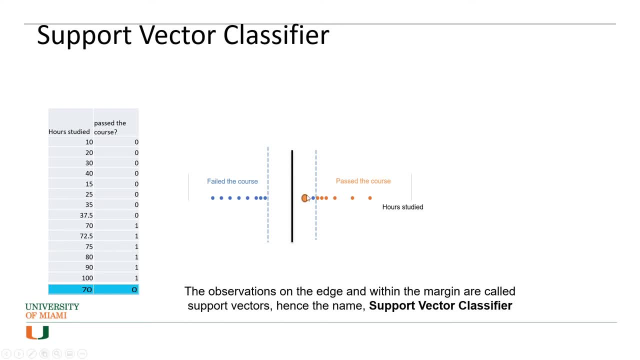 right, the classifier is going to change only based on the changes of the observations to the uh at the margin right at the very edge of the two groups. now here the million dollar question is okay. how do you decide, uh, what margin of error to allow your support vector classifier to have, basically, how far away from the center line you would? 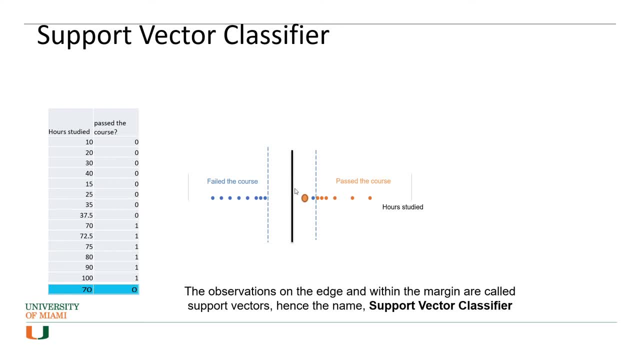 allow the margins to go? or how wide are you going to have? uh are you going to have for your street right that you're running through this, because you know these dotted lines could be way closer to the main uh middle line, or they could have been way uh farther away. well, that is uh going to be uh decided based on cross validation. 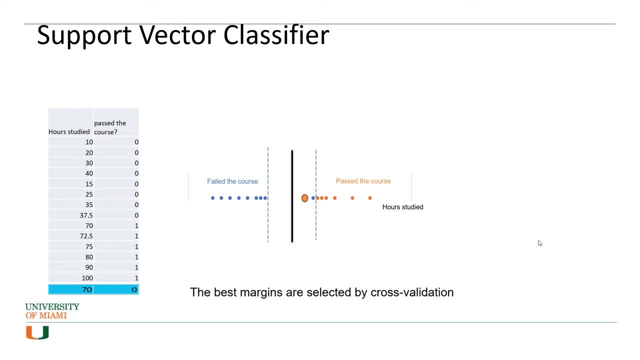 and that is basically a tuning parameter for your uh, for your uh support vector classifier. it gives you a lot of flexibility on uh, on determining that particular parameter uh, and seeing how well your algorithm makes predictions. so so that is up to you. but before i show you how you can actually 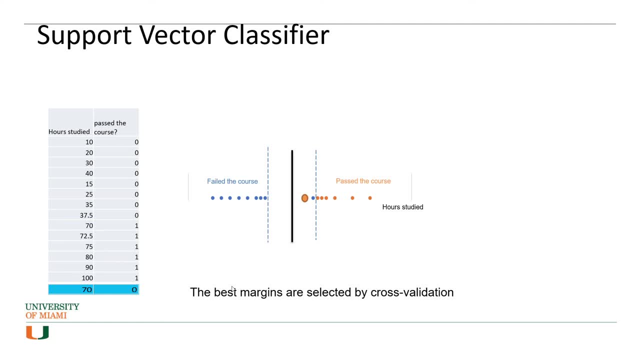 go ahead and and choose that tuning parameter, how you are basically going to find the best margins based on cross validation. let me show you the mathematical problem for support vector classifier, and then it would make it much easier to understand what the tuning parameter is and how the cross validation works. well, uh, the, the formula is: 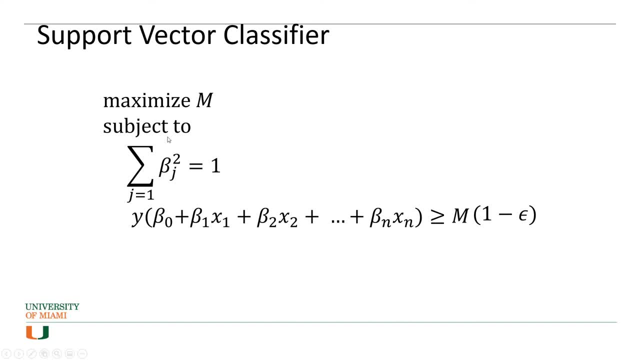 actually very uh similar to what we had uh for uh maximum margin classifier. so here again you have the distance, uh, and you are going to maximize the distance uh, subject to uh the constraint that the beta j's uh squared should be equal to one and uh the distance should. 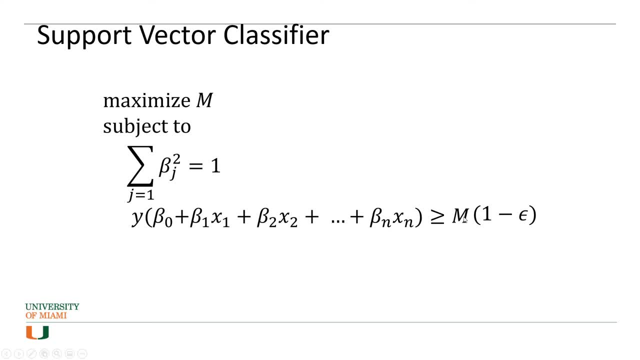 be larger or equal than m. the difference here is that, uh, we are allowing some error, uh, so we're here. we can say the distance should be larger or equal than m multiplied by one minus epsilon, in which epsilon is a non-negative value. so we can say the distance should be larger or greater than zero and the sum of the epsilons. 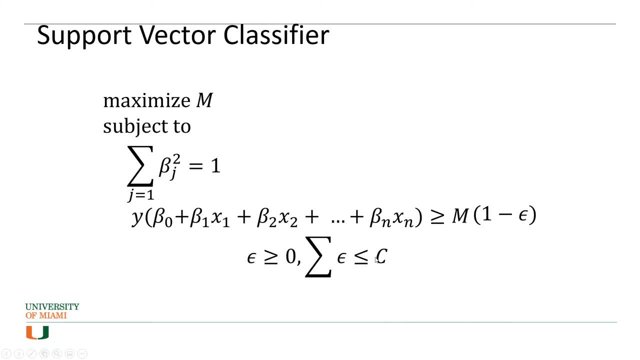 for all the observations in your data set should be less or equal than c and, depending on how you choose this c, how large you choose this c, you are allowing uh more errors, or you are uh you are widening the margins for your tube or you are widening the street that you are. 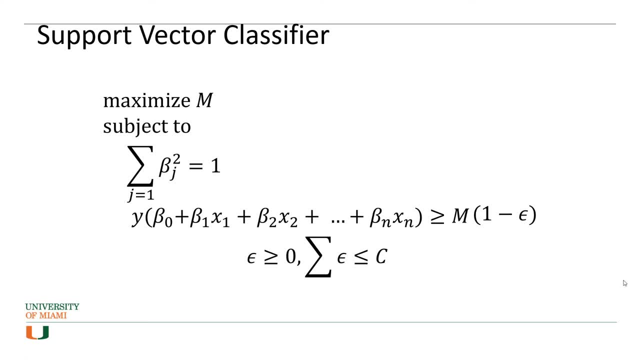 you are running through your points so you can imagine at the extreme, where epsilon is chosen to be zero, you are allowing zero misclassification. right, the margin is actually set equal to zero and this will turn out to be the formula for the maximum margin classifier, because one minus zero is equal to one, and one multiplied by m is equal to m right now. on the other hand, if 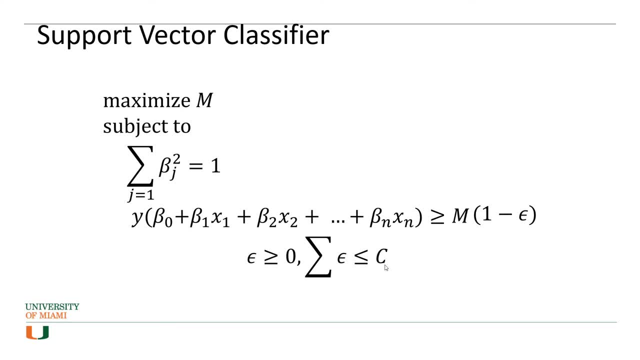 you start gradually increasing the value of c such that, uh, the corresponding values of epsilons for the observations is is- is going to be allowed to move away from zero and become larger. you're actually moving the margins from the middle line to the right, to the right and to the left, allowing 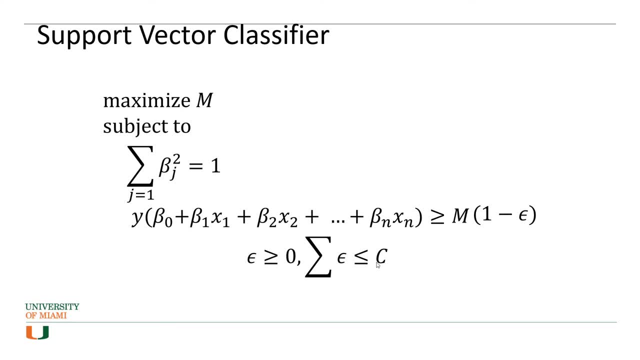 more misclassifications. now the point is: okay, how are you going to choose c? what is the best value for for the c? and i said that you would choose that based on cross validation. so what does class? uh, what does cross validation mean? suppose that you have a data set. i'm showing 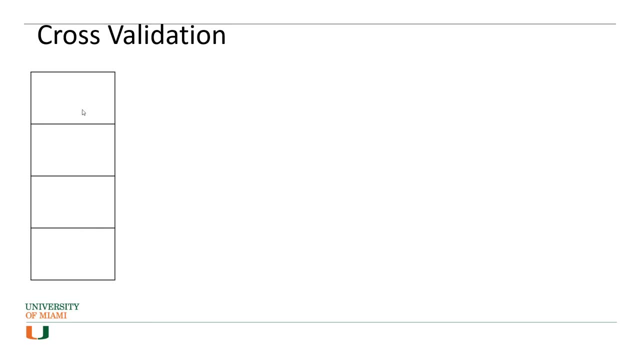 it, uh, you know, uh, demonstrating it by, by this. and usually you choose a proportion of your data set for training and another proportion for testing. so in this particular case, suppose that we chose the for training and the blue part for testing, the. the point is that you do not necessarily have to. 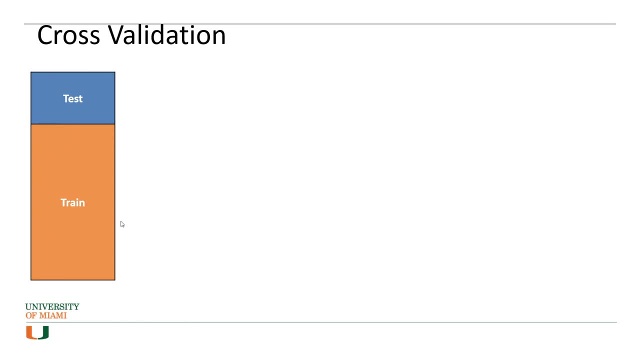 choose these specific observations for training. you could have chosen other observations, but once you choose a specific set of observations for your training, you can have a particular accuracy measure. and then, if you choose another set of observations, you say that here you're again going to choose seventy five percent of your observation for training. 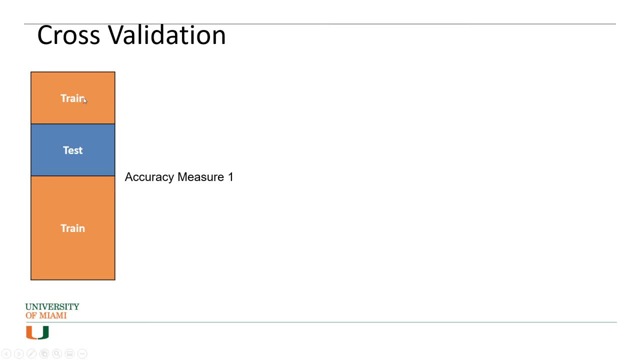 but they are going to be a different set of seventy five percent of the observations and you're going to choose twenty five percent for testing, but they are going to be a different set of observation for testing. that will give you another accuracy measure and you can continue. 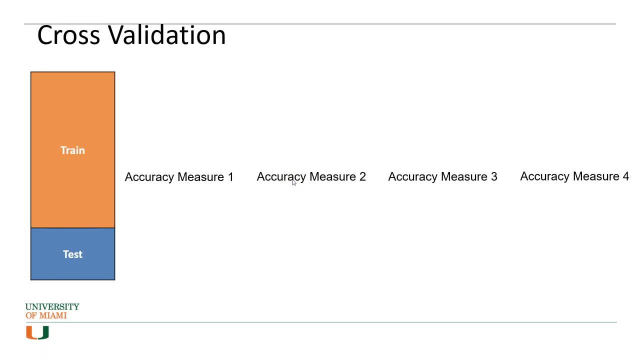 doing it depending on how many folds you are going to create in your data set. in this case, i'm going to say that it is a four-fold uh cross validation. so i am going to choose four different uh sets of training and testing and i am going to calculate four different accuracy measures. 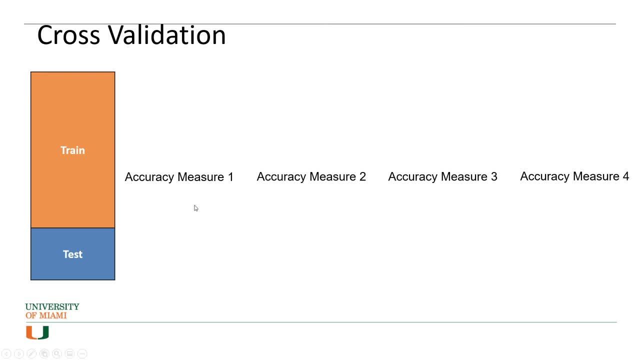 and then i am going to find a way to summarize all of these accuracy measures together. in this case, i take their average, and that would be my overall accuracy measure. so this is how the cross validation works: uh in order to choose the. uh- in order to choose the value of c: the. 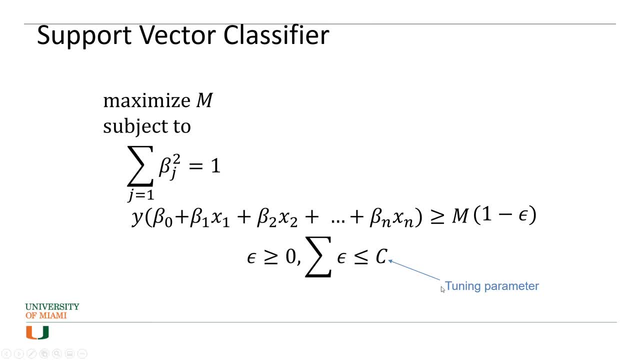 training parameters. what we are going to do is that we are going to choose a random value and then, uh, do cross validation. meaning that, given that particular value of c, we will see how well our model does overall right. meaning that, how well our model does when we choose many different. 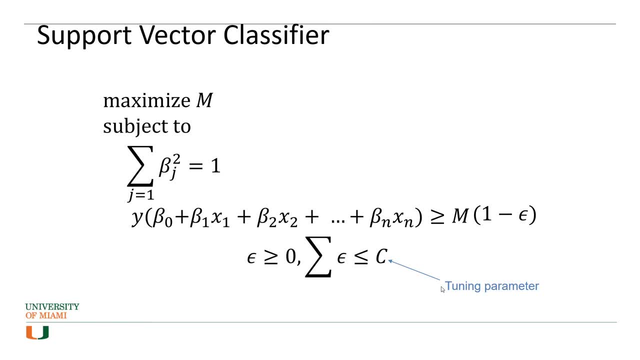 combinations of training and testing data sets and calculate an overall accuracy for the performance of our model when it comes to testing. given that value of c, right, we record that, and then we are going to choose another value of c and see how well the model does, again overall, based on different combination of training and 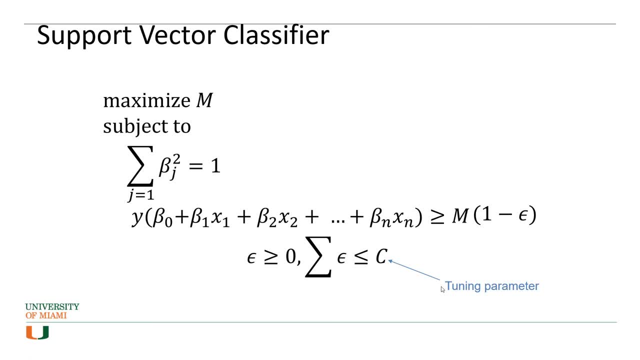 testing of of the data set. and we, we continue doing that and we continue calculating the overall accuracy measure and recording that, and then we're basically going to see: okay, what is the value of c that is going to give us the best performance? all right, these support vector classifiers work. 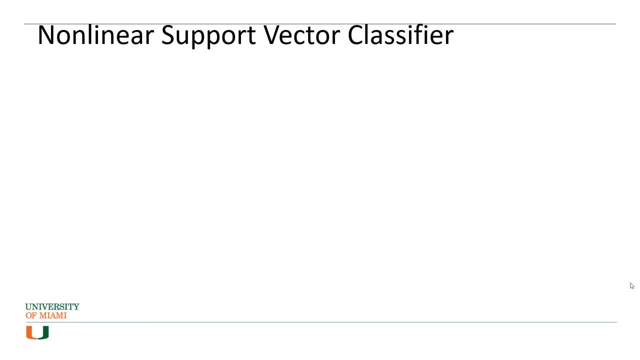 very well. well, when you can find a straight line or a hyperplane or a point that can go through all the lines and very cleanly classify them into two classes. however, that is not always uh the the case you. there are many situations in the real world where you cannot have a linear line. 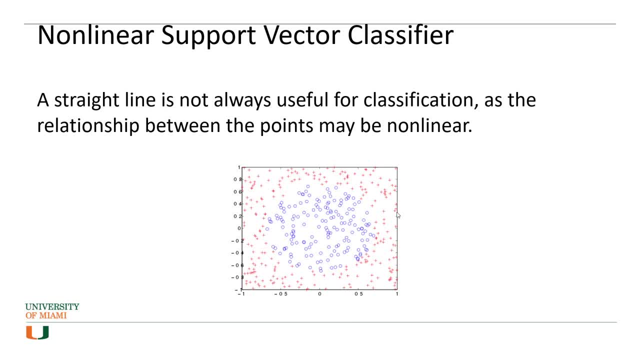 separating the observations. this is an example, right, so you can have a situation where you want to classify patients into the ones that got better after taking a drug or did not get better after taking a truck a drug. so there you have two classes. you know, uh, got treated or not. 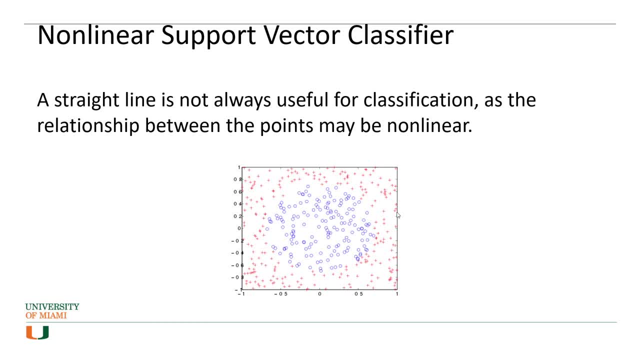 and the uh features that you have is the amount of dosage, basically the dosage of a treatment that they receive, and there are many cases where, if they have received less than a certain dosage, they wouldn't show any results, and there is a there is a range of dosage for that drug. 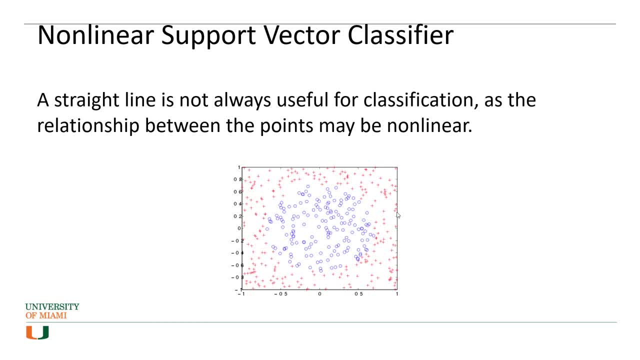 that if they take it they would do better, and anything more than that would actually adversely affect their situation. right? so you're going to have a situation where only between a minimum and maximum of dosage you will see reaction- positive reactions to the drug, and anything less or anything more does not work right. so in that case it's very difficult to come. 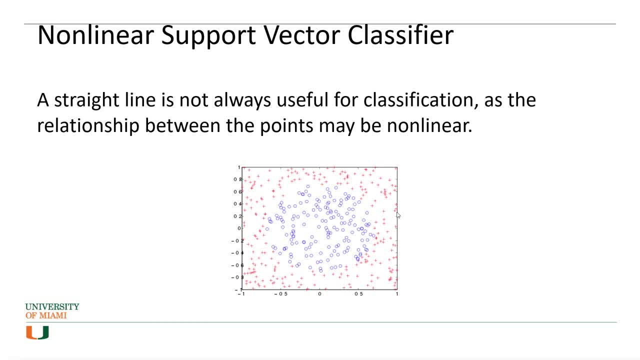 up with one point that you can say: anything less than this or anything more than this is going to be in either of the classes. here is the two-dimensional example. here you can you can say that if you have two features and then the classes are with the blue dots and the red crosses, it is. 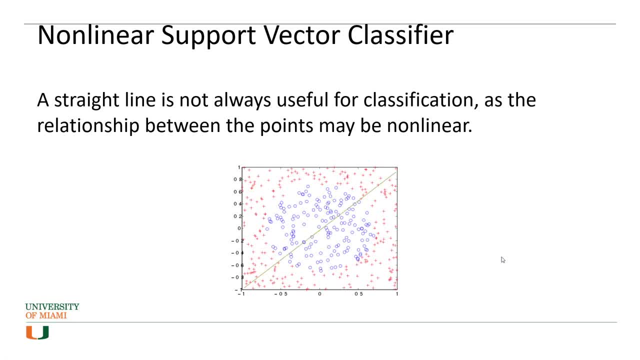 impossible to find a line that can uh, that can uh, classify these observations uh appropriately right. so what is the trick? uh, and actually the the best uh classifier is something that resembles an, an oval, or like a, like a circle, right, it is completely non-linear and the the question is how. 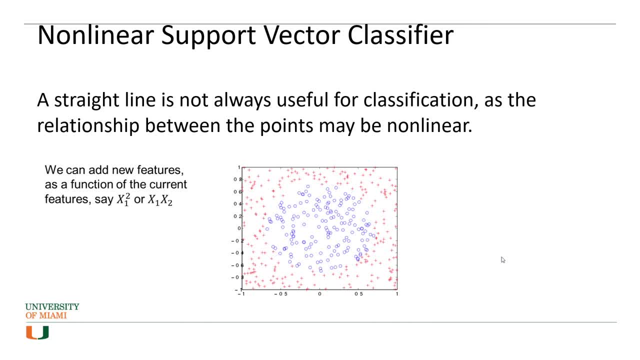 to find that well, if we can add a new feature based on a combination or polynomials of other features, say x 1 square or x 1 multiplied by x2, then we can move this from a two-dimensional space into a three-dimensional space like this and then run a hyperplane that perfectly separates. 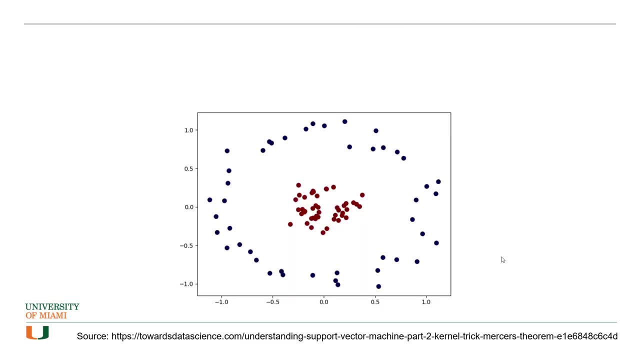 the blue dots from the red crosses. here is a example of it. I took this from the TORS data science website. You can see the link below if you want to read the article yourself. But if we have a two-dimensional space, you know we have. 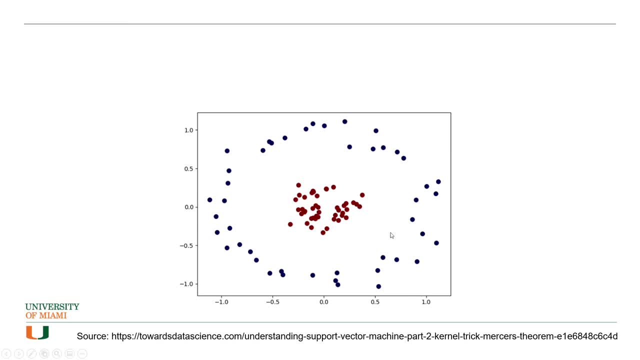 features X1 and X2, and these are the groups. In the middle we have the red group and all around it we have the blue group. We cannot separate them. However, if we come up with a third dimension, let's say based on X1 multiplied by X2, then we can bring the red dots. 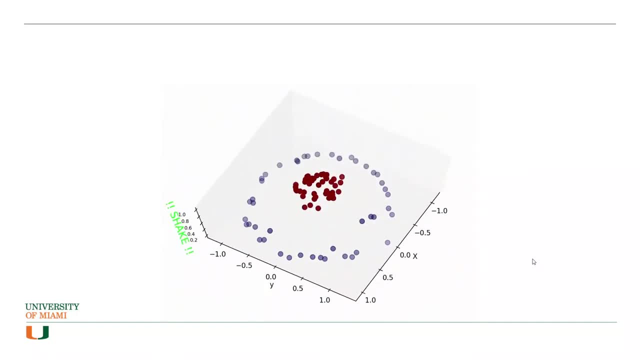 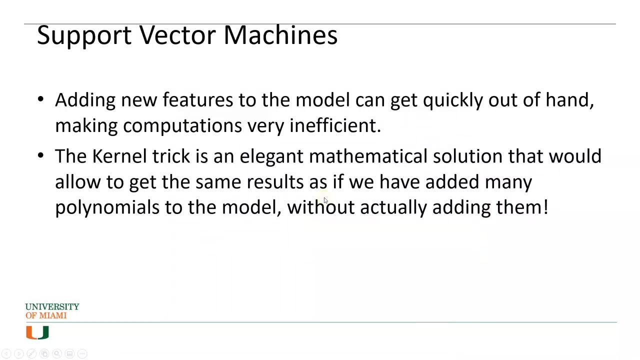 lower and then run a hyperplane right in the middle in a three-dimensional space here and basically separate these two classes quite perfectly. So that would be the nonlinear dimension support vector classifiers that we have. However, as you can imagine, adding new features to the